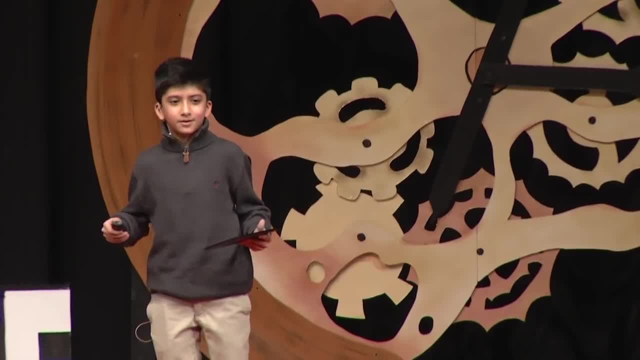 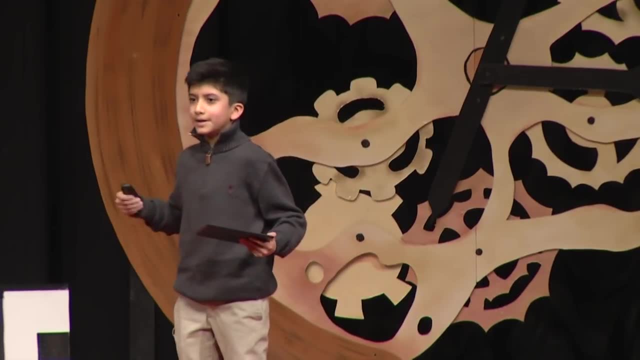 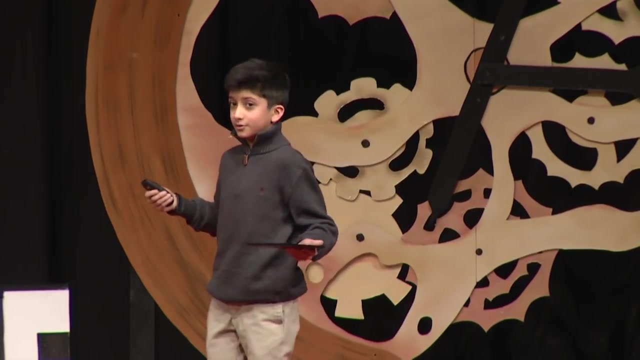 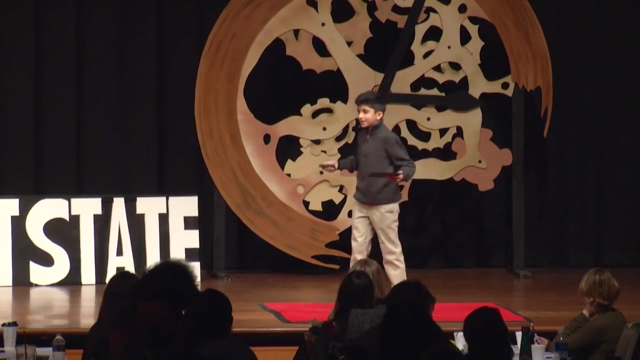 so most people will follow up and ask: what is coding? My answer to this is: coding is based on many different languages that computers understand, just like how you and me can speak English and understand it. But the real reason I'm here isn't to educate everyone on what coding is. 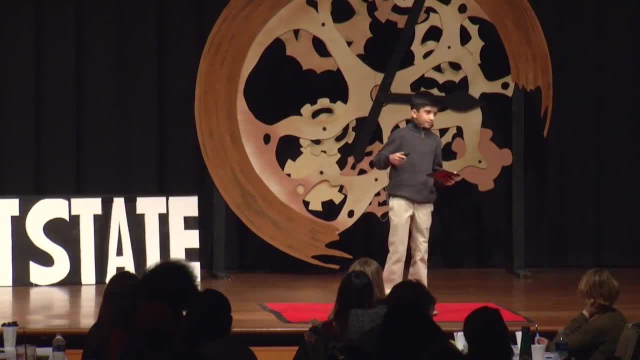 but to address a problem. Most digital things we do involve code, but only a small percentage of the world actually knows how to code. For example, how many of you have searched something on Google? Yeah, probably every single one of you. Or how many of you have bought something online? 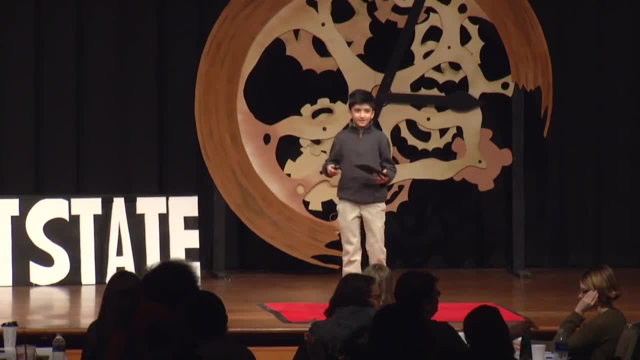 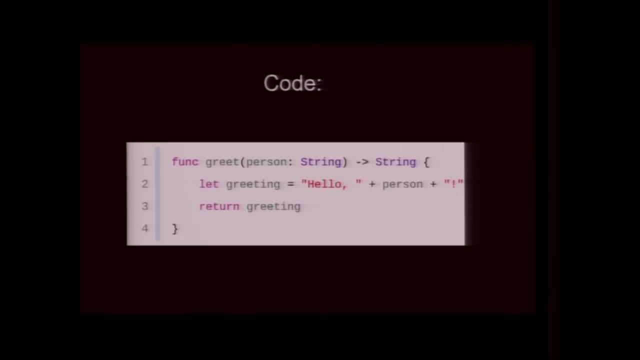 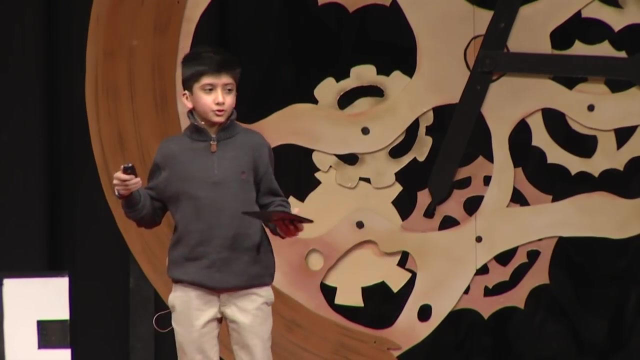 Probably every single one of you. And well, what the heck? Okay, That's a snippet of code, and you're probably thinking that that's really complex, unless you know the Swift coding language or anything similar to it- And I did too before I started coding. But the truth is it's not complex. 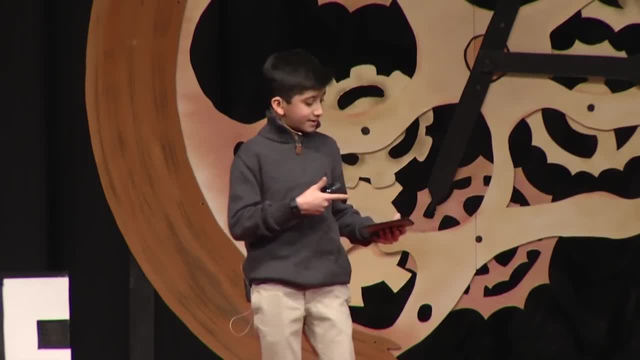 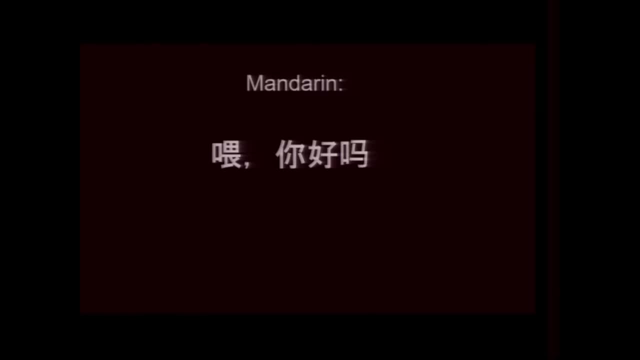 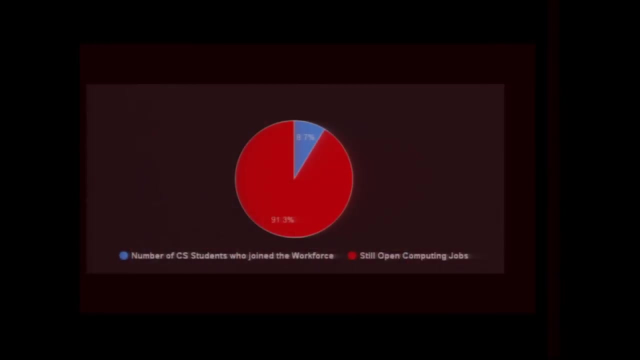 Wouldn't you also think that that's complex, Even though it's Mandarin, the most widely spoken language in the world? So last year, according to Codeorg, 43,000 computer science students graduated into the 494,000 open computing jobs. 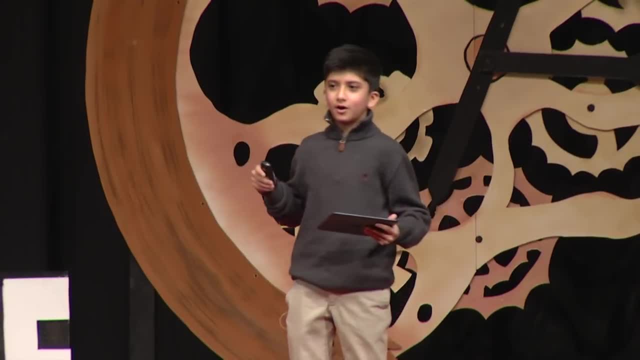 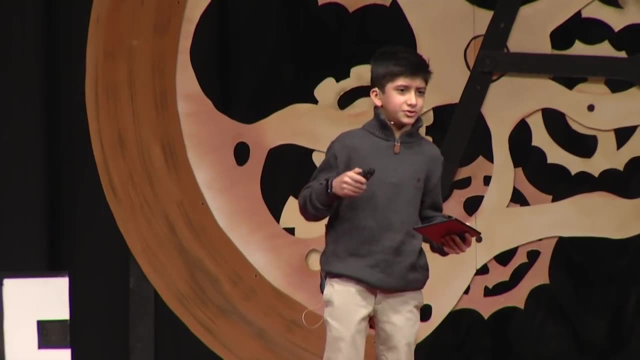 If that wasn't clear enough, there were still 451,000 open computing jobs. According to International Data Corporation, also known as IDC, only 20% of computer science students graduated into the 494,000 open computing jobs. 25 out of every 10,000 people know any code in the world. 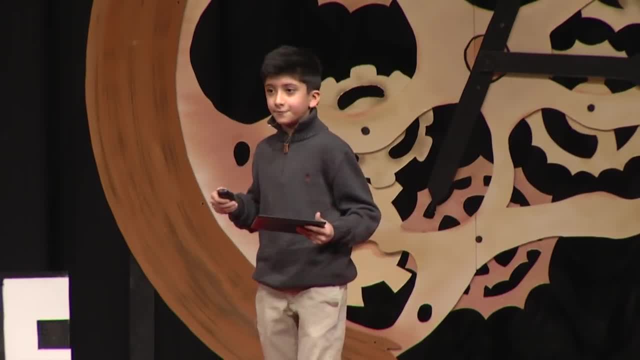 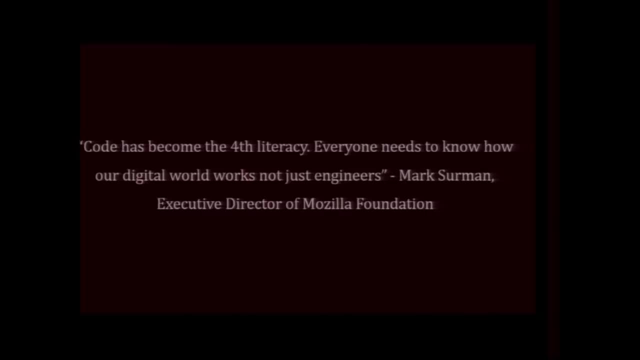 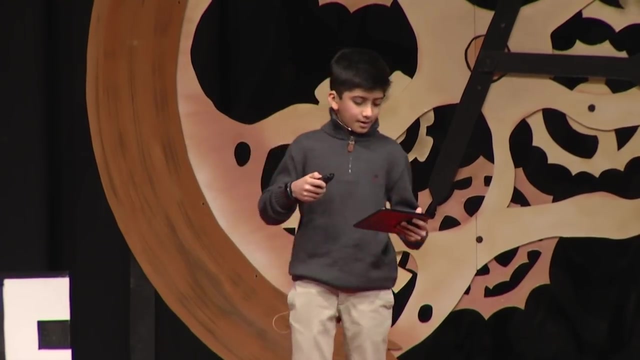 Code has become the fourth literacy. Everyone needs to know how our digital world works, not just engineers. Mark Sermon, executive director of Mozilla Foundation, said how many of you have changed a light bulb? I'm guessing the fair majority of you. 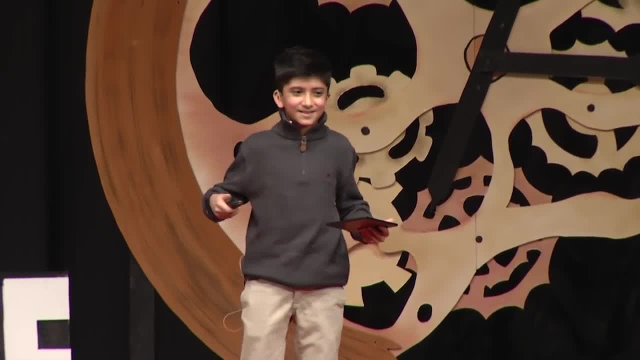 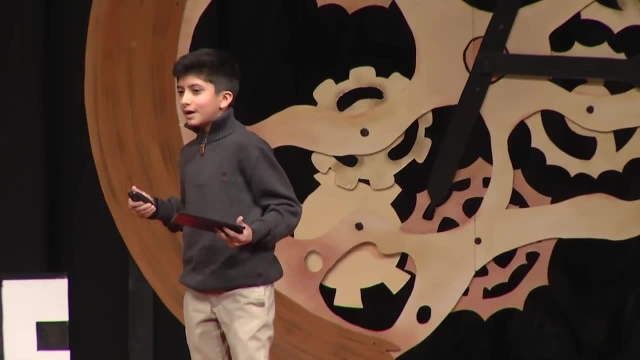 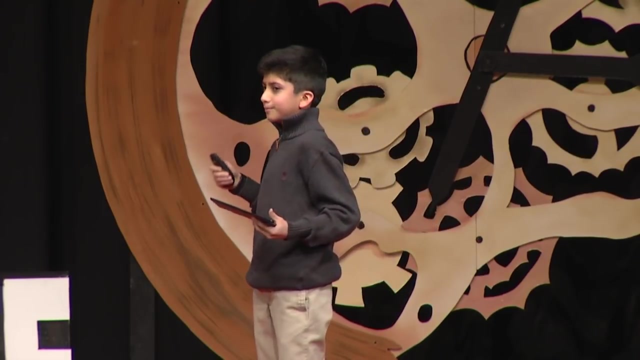 But are we all electricians? Probably not. This is just like coding, because even though we should all know how to function a computer and write simple lines of code, it doesn't mean that we're all going to be computer engineers or computer scientists. 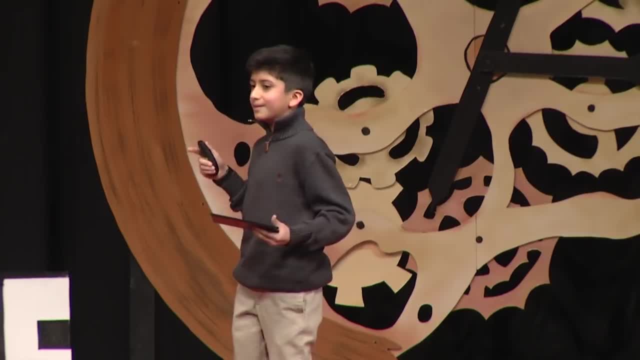 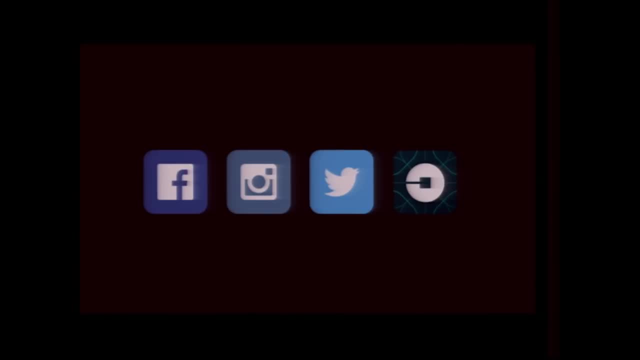 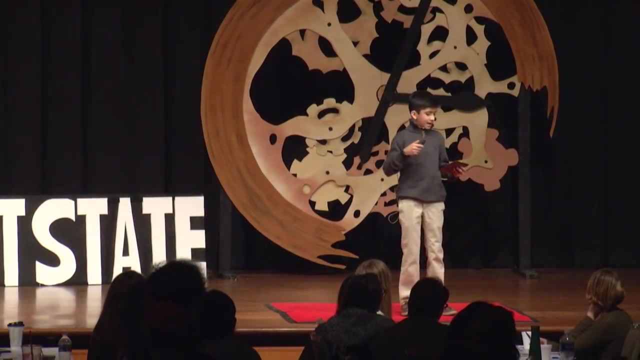 As we speak, coding is becoming more and more important to us. Facebook, Instagram, Twitter and Uber are all examples of how we are coming to depend and rely on technology more than ever. Imagine how much we could get done in the next few decades. 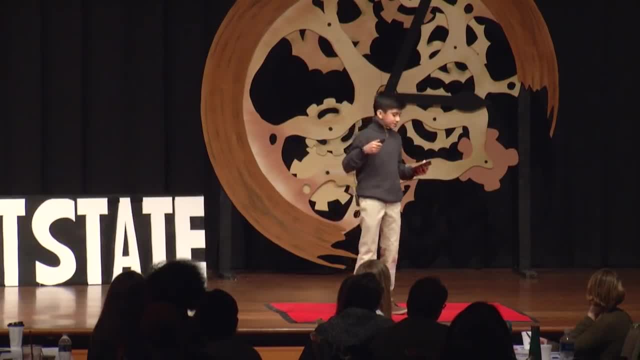 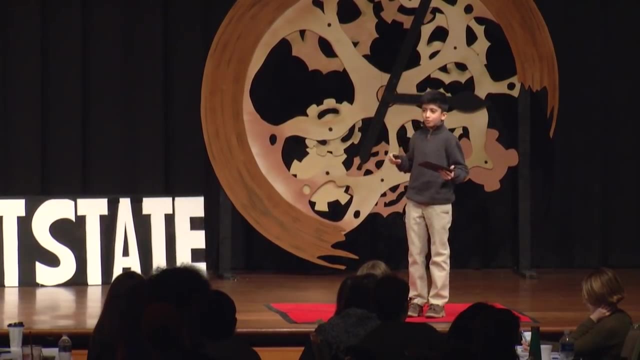 if every kid right now learned even just the basics of code. When I say this, I don't only mean kids that live in wealthier countries, but I'm also talking about kids that live in developing countries such as Brazil, Nepal or even in the United States. 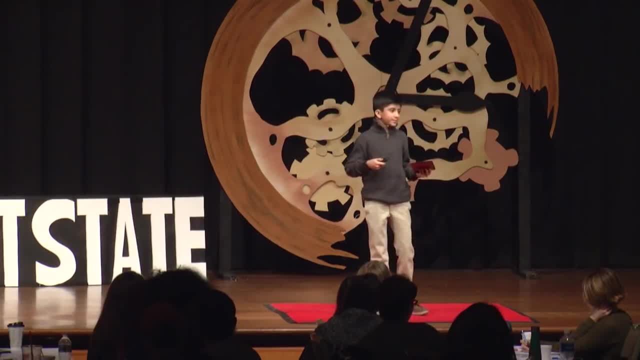 Or even Kenya. By this point in my talk, you're probably just wondering how to get your students or children started coding. Implementing coding into curriculum would definitely spark interest in coding for students. This is because they would finally get to use all of those ideas. 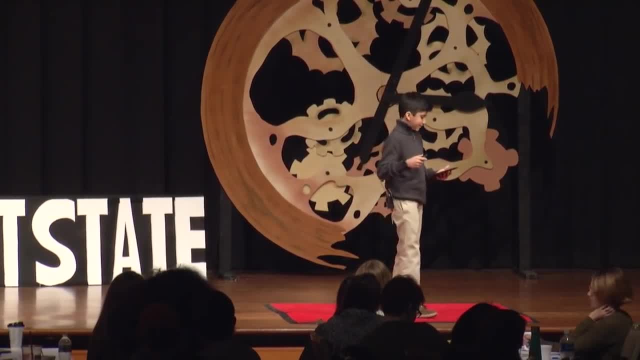 that just sit in the back of their heads the whole day And they would get a break from what most of them think of as boring classes. and I have to agree. To spark interest in coding at my school, I started a coding club. 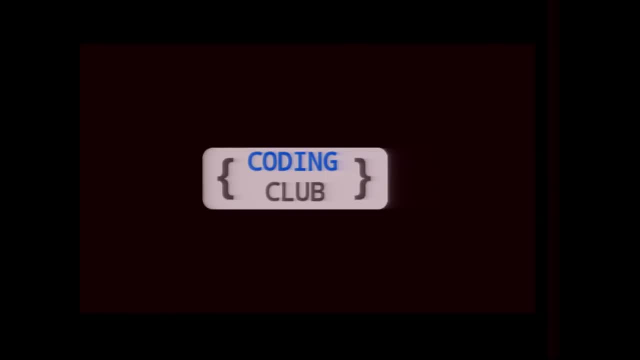 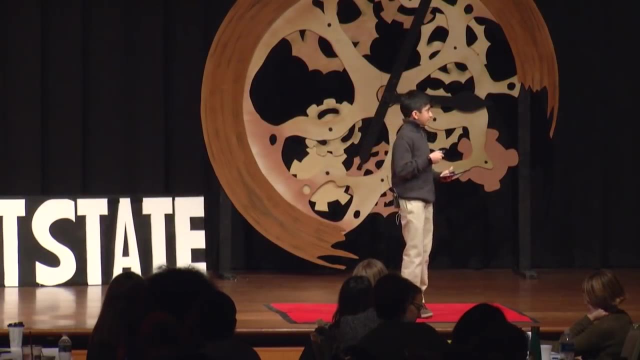 At my coding club we are teaching simple coding and letting kids use their ideas to the fullest. In my case, coding is kind of like soccer or tennis, Because in both sports if you make a mistake you can work to fix it. 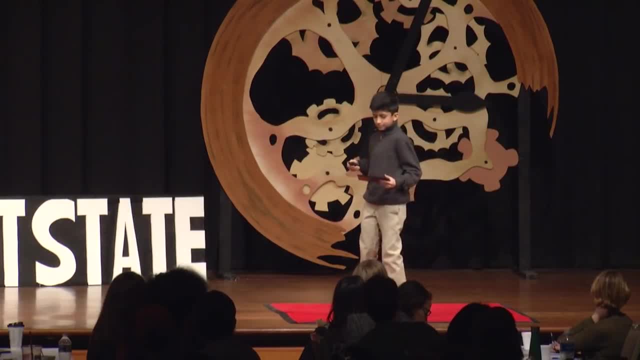 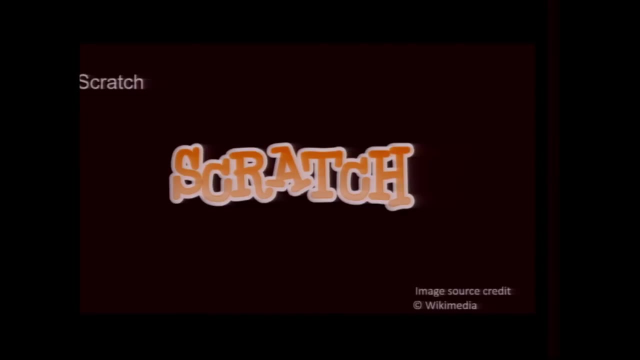 Just like how you can in coding. Now I'm going to list some places that you can get started coding. To start, there is Scratch. Using Scratch, you can create games cards and utilities using simple drag-and-drop blocks. Next is Code Academy.